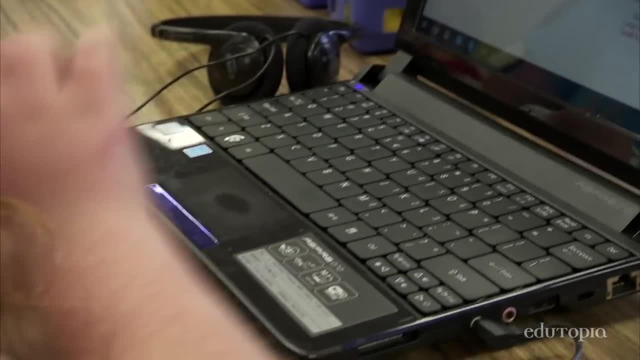 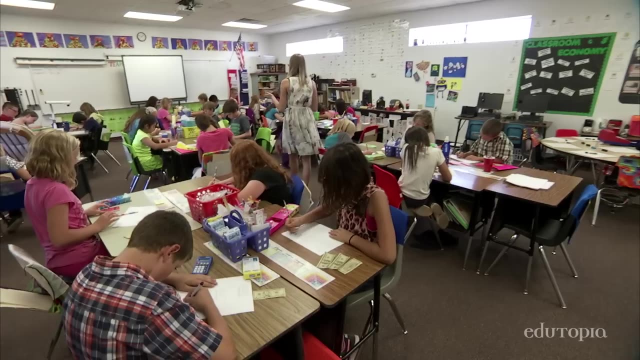 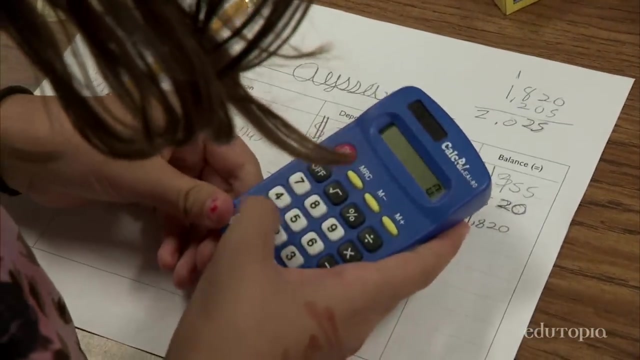 during that last 30 minutes. They have specific skills that we're trying to progress, monitor, benchmark and move them forward with. So in my classroom the kids at the end of our math lesson have a formative assessment and it's usually four questions and it covers the concepts that we did that day And I grade 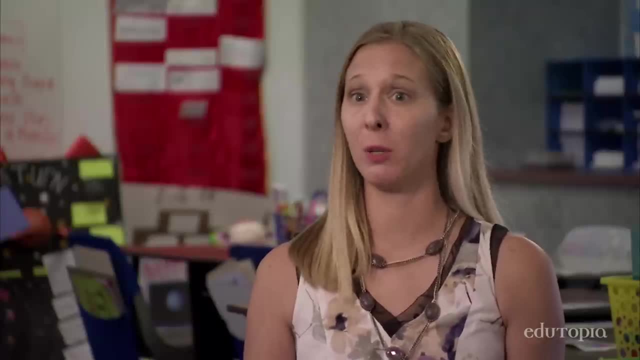 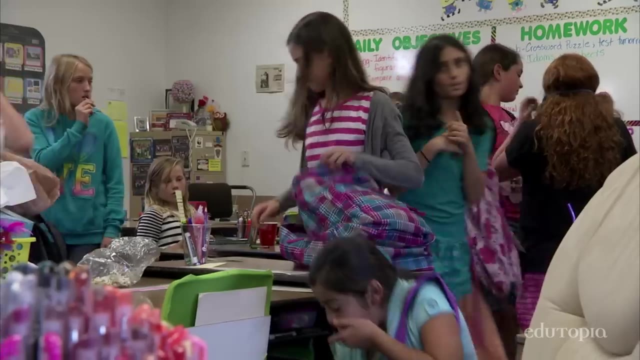 them very quickly and I am able to determine who understood what we were doing that day and who didn't. So the kids that got usually an 80% or higher, they go to their. I choose for that day The kids that didn't. 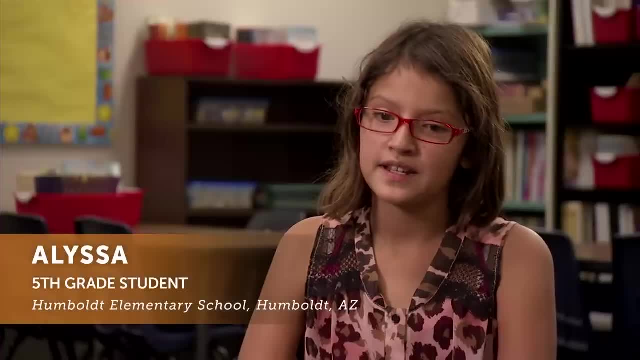 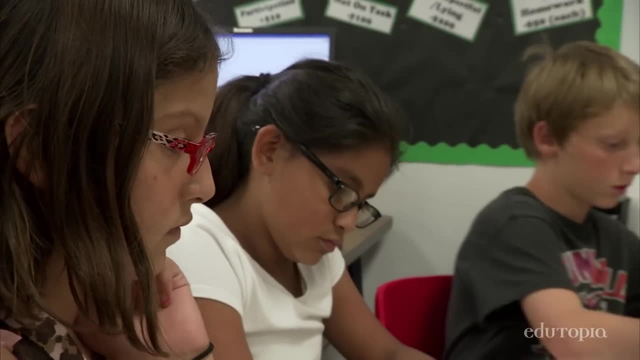 Will stay here with me. We do a pre-test and sometimes if you get one wrong, she helps you on it. Okay, so I'm here to help. We're going to play some blackjack. Poker face is on. okay, Poker face is on. 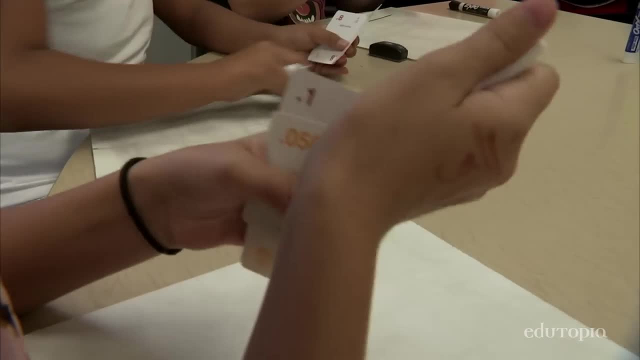 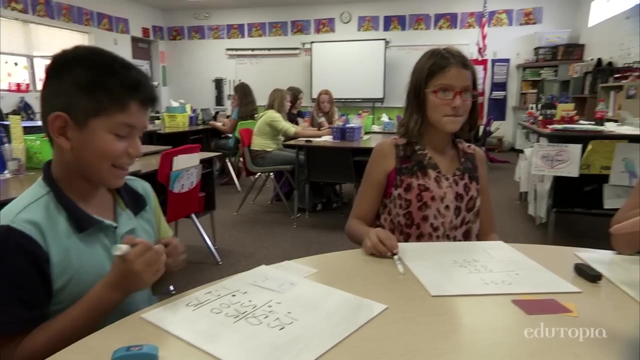 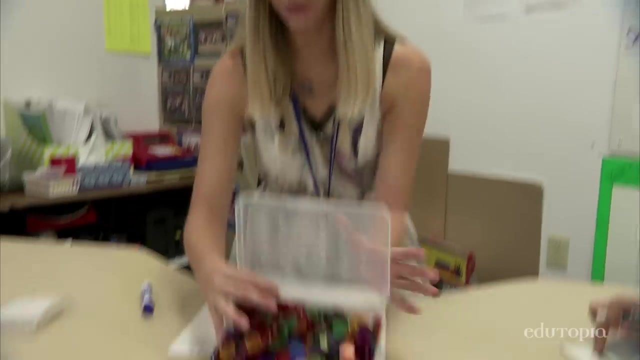 And we usually just go over the same lesson over again. I take out the manipulatives. we play games. It's visual for them in kinesthetic, But we have 951,000.. Can we give her a round of applause? She's definitely closer to one. 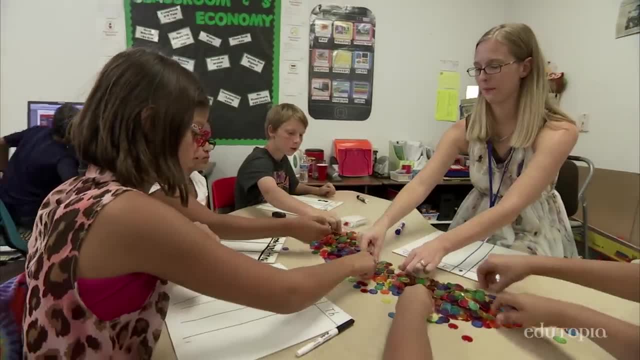 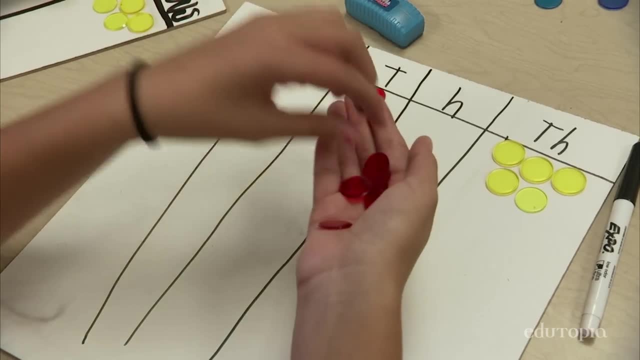 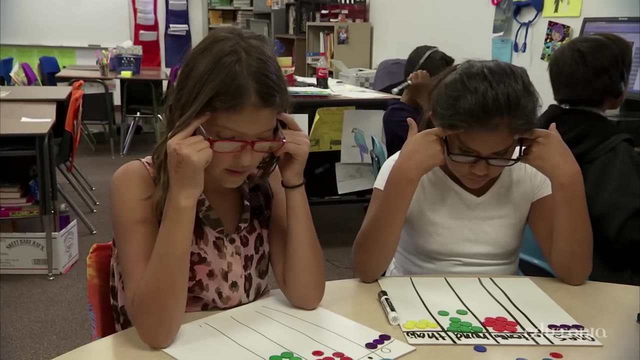 Last time I didn't get the decimals right. She helped us on the homework part and she taught us how to do the decimals in an easier way. And I want you to think right now: how would I say this number? The teacher head shoes is actually a great time to close those skill gaps and make them. 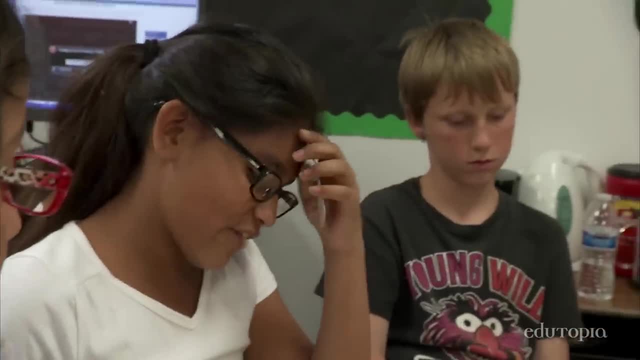 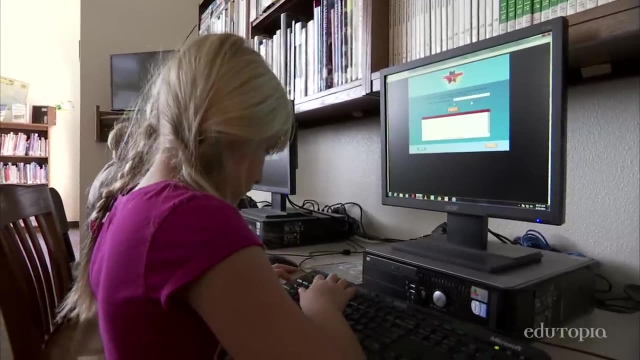 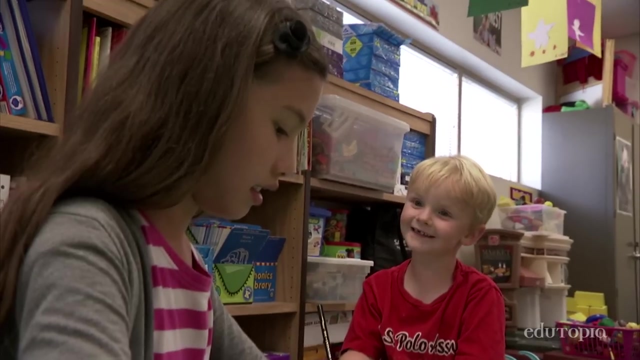 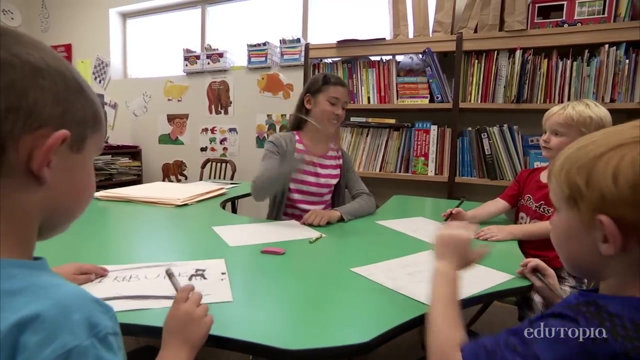 proficient and make them successful, which makes everyone happy. The ebb and flow of iCHOOSE changes every single day, based upon not only the performance but also how they did in class and what the teacher feels is best for the child. We even have kids in fifth and sixth grade who take their half an hour and their iCHOOSE. 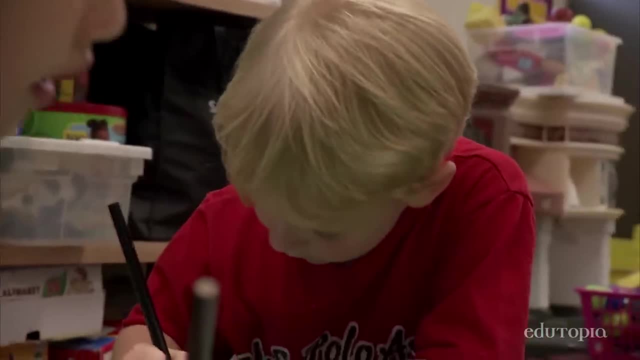 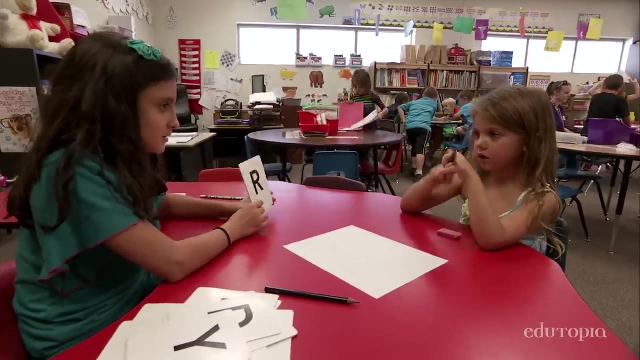 is going to help out first graders in the RTI process, whether that's doing flashcards to help them with their sight words or letter names or whatever. The teachers are happy because they were the push for it. They were the ones that wanted the time. We were able to find it for them.